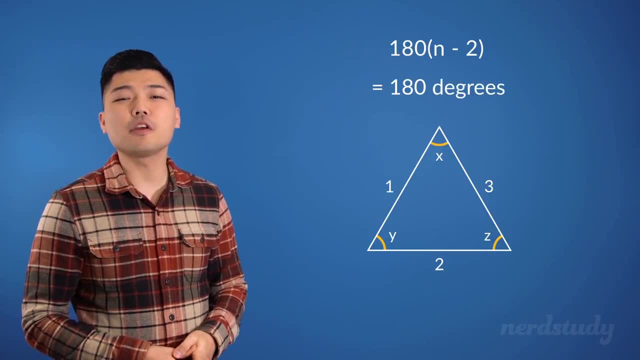 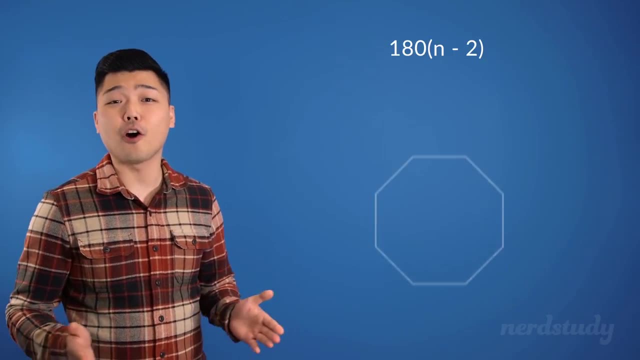 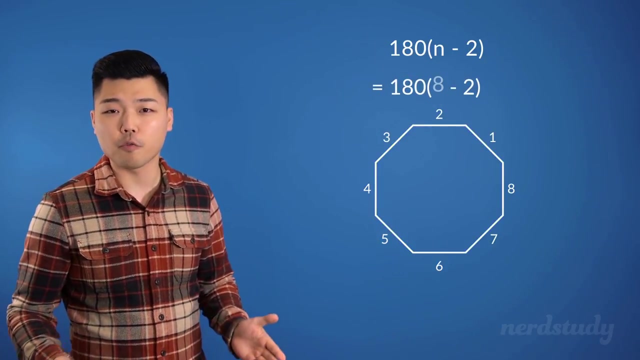 which is 1.. And thus the sum of all interior angles in a triangle is 180 degrees. Alright, and what if we take an octagon as an example? Since it has eight sides, all we'd have to do is plug in 8 into our formula. 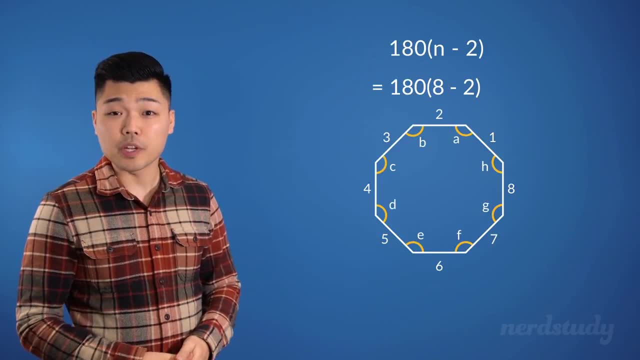 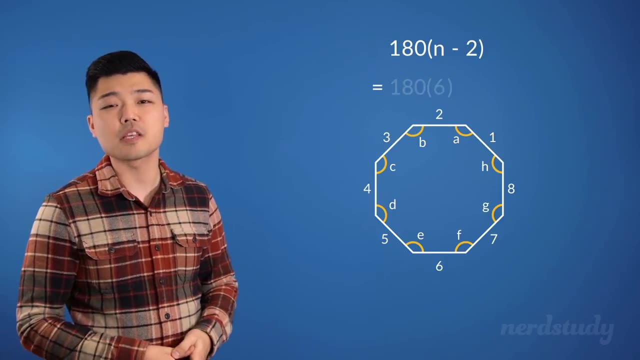 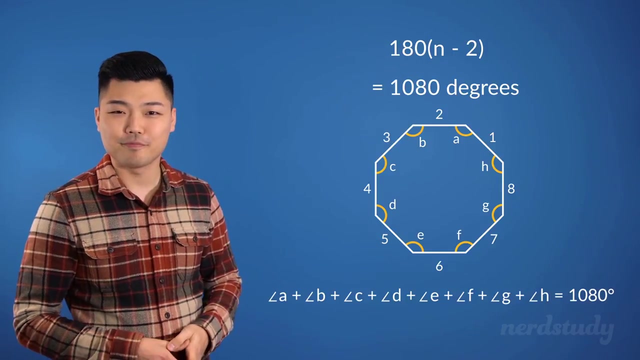 for the sum of all interior angles and we'd get the following: 8 minus 2 is 6, and 180 times 6 gives us 1080 degrees for the sum of all interior angles of an octagon Great, So just remember that formula. 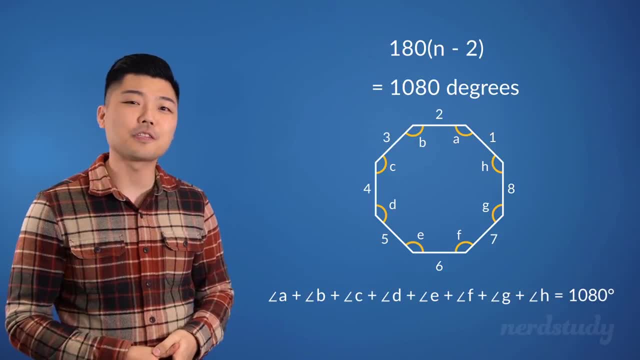 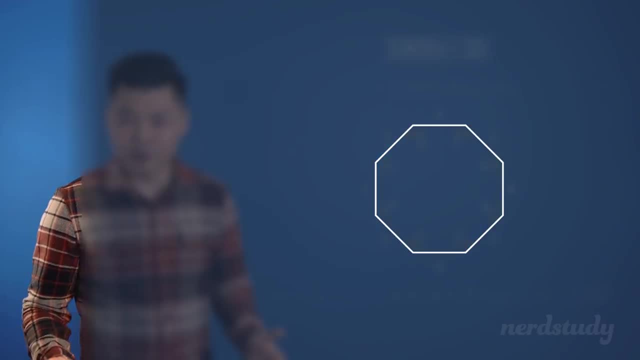 The sum of all interior angles in a polygon is equal to 180 times n minus 2.. Now, what about the sum of all exterior angles? Well, I'm pleased to tell you that, regardless of how many sides there are in a polygon, 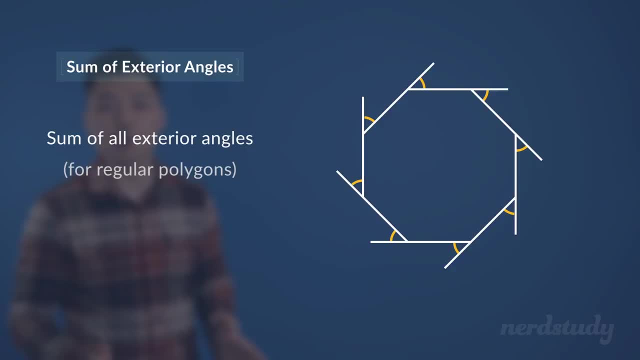 the sum of all exterior angles is always going to be 360 degrees, And that makes solving questions really easy. But let's think about why. Let's think about this octagon and start off with one of these sides. This exterior angle here can be seen as the amount that is turned. 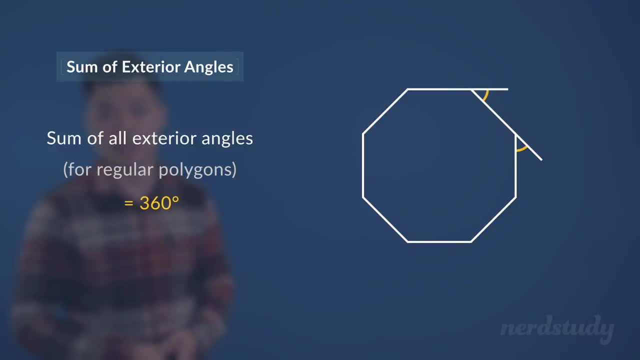 in order to reach the next side. And again, the next line is turned, yet again by however much the exterior angle is, which is this way In order to reach the next side of the polygon. You can think of the exterior angles as the amount that these lines turn. 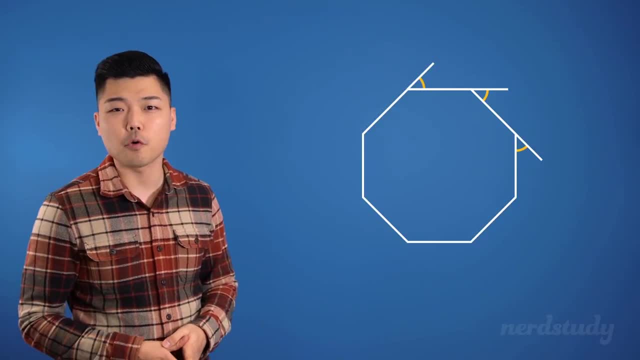 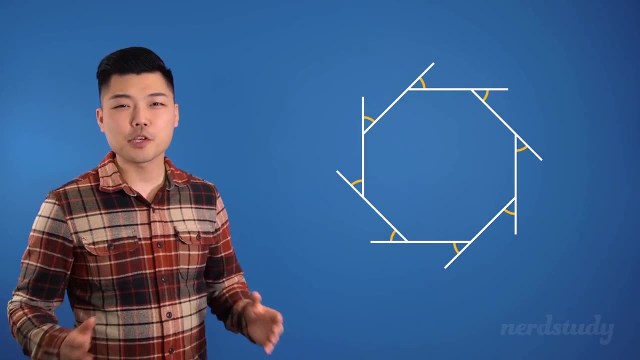 in order to get to the next side of the polygon. Of course, if we keep doing this turning, then we know that we would get back to where we started from. So if we take a step back and think about it for a moment, 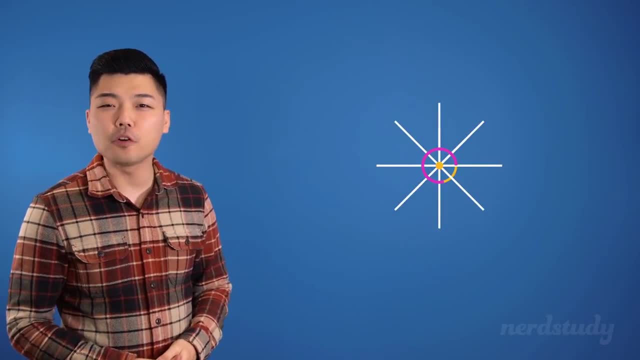 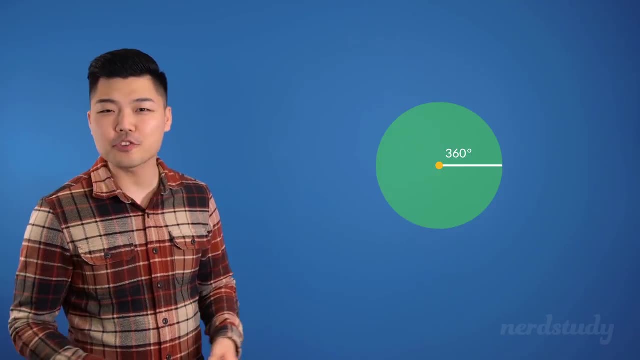 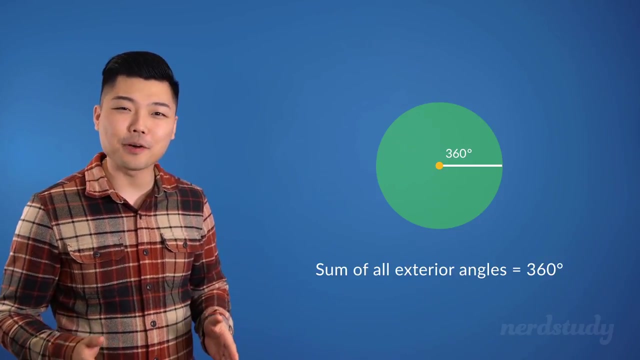 all of these turns add up to be one full rotation, Doesn't it? And a full rotation is the same as a full circle, which is 360 degrees. So it makes sense, then, that the exterior angles of a polygon would add up to be 360 degrees. 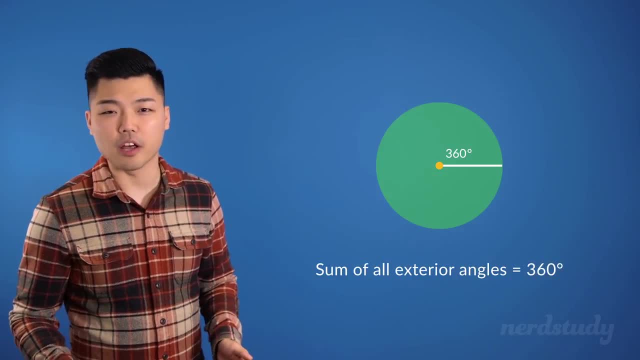 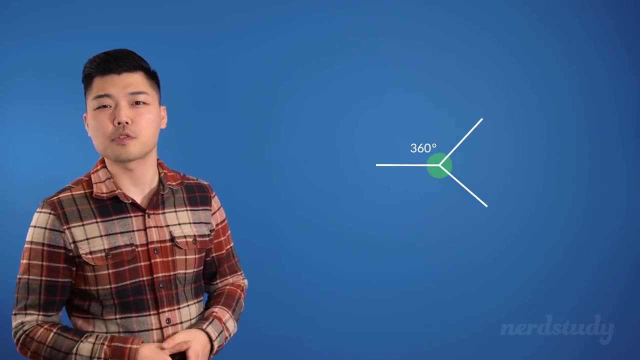 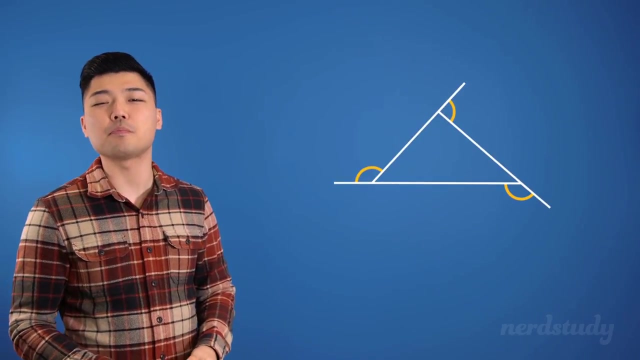 And even if we had less sides to this polygon, for example three sides like a triangle, then there would just be less turns, so to speak, making each angle a bit larger, which results in the exterior angles to add up to be 360 degrees yet again. 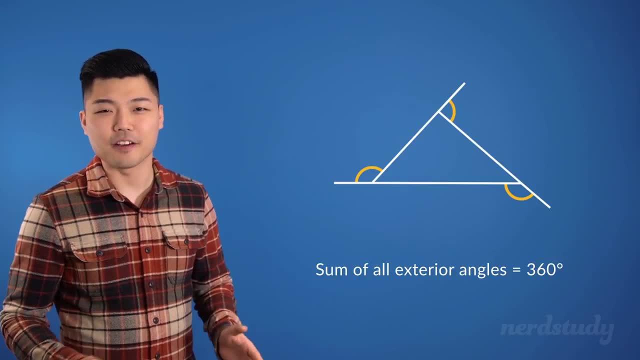 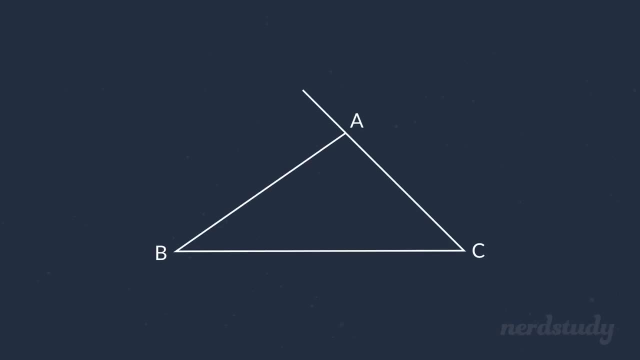 Awesome. So let's try an example together. now Imagine that we have a triangle ABC where the angle ABC equals 35 degrees and angle BCA equals 45 degrees. What would the exterior angle of X be? Well, we know that a triangle adds up to 180 degrees, no matter what. 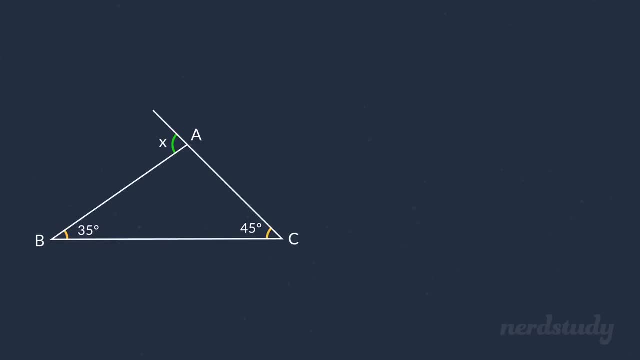 If we haven't memorized that by now, we know that we can always use our formula 180 times n minus 2, and we'd get 180 times 3 minus 2,, since there are three sides in this triangle. Simplifying this gives us 180 times 1,. 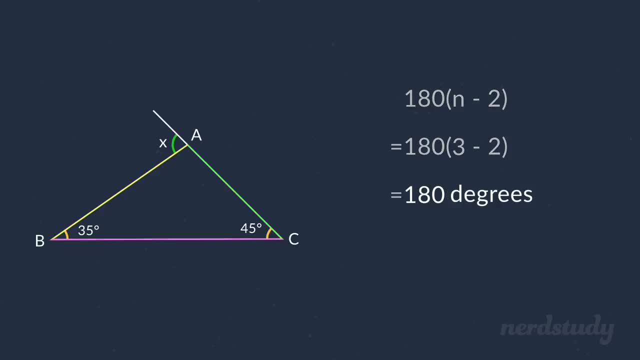 which is just 180 degrees Great. And since we have the values of two of the angles in this triangle, we know that this angle over here would just be 180 minus 35 minus 45. Computing this gives us 100 degrees for this angle. 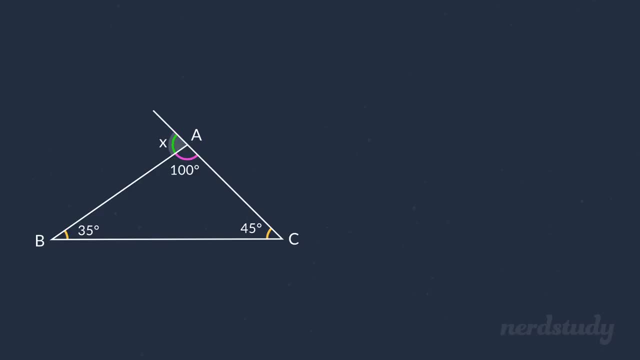 Finally, to solve for this exterior angle, we just learned that an interior angle plus an exterior angle equals 180 degrees. So again, we do 180 minus 100 to get 80 degrees. Therefore we get 80 degrees as our exterior angle here. 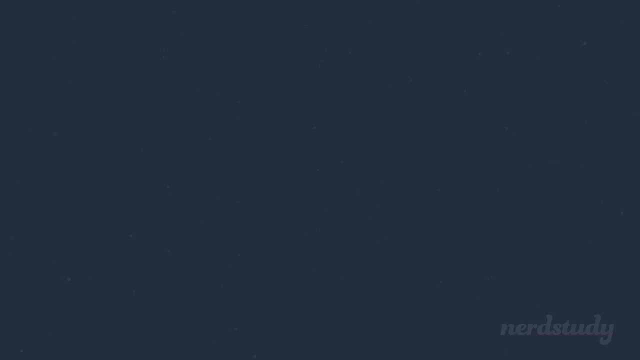 Awesome, So let's just try one last question before we end this lesson. In this question we're given the following information: In the triangle ABC, the sum of the exterior angles of angle B and C are 210 degrees. What is the value of angle A?